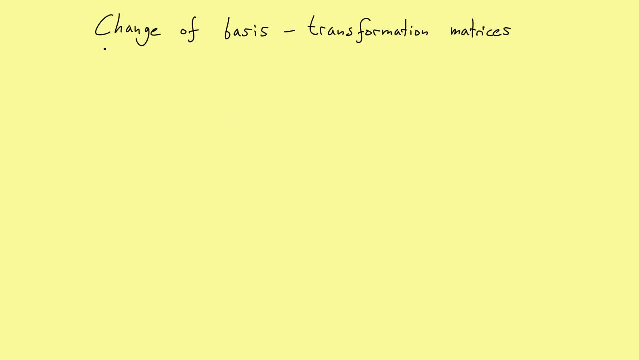 Hello and welcome to linear algebra. Today I talk about the change of bases, and related to this are transformation matrixes For better visualization. I will do this for the vector space R2.. So we have a two-dimensional vector space. We can see this vector space just as this plane, and so we have an x and y. 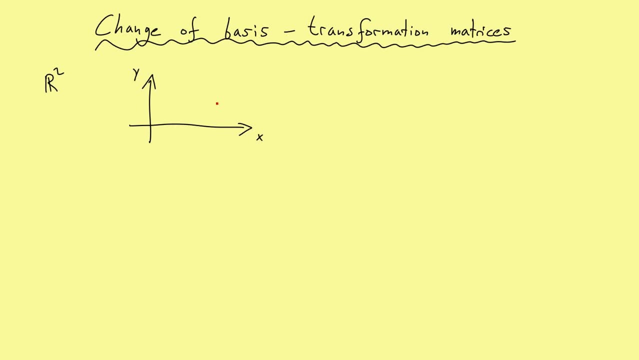 coordinate here and for each point here we have a vector error that goes to the point. So we can imagine these vectors just as a set of these errors. Usually we can describe such an error just by saying how many steps we have to go to the right in the X direction, and how many steps we 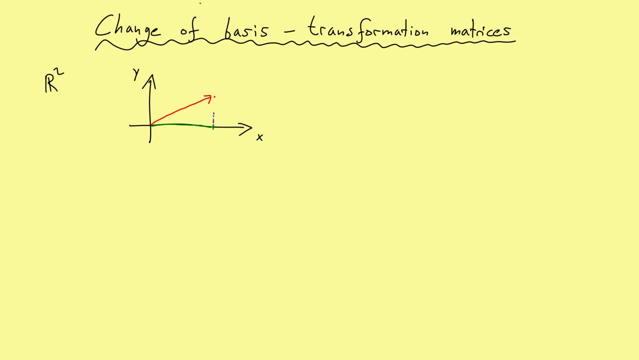 have to go to the left. Here you can see that the where and the where are all have to go upwards in the y-direction. So for example, here we would have four steps and three steps, for example, and the vector arrow. here is just four in. 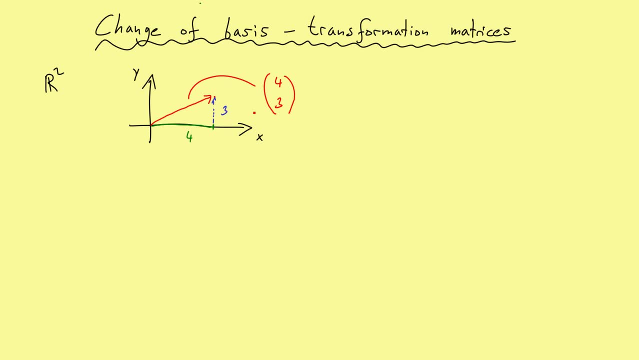 the x-direction and three in the y-direction, And this already means that we have chosen the basis of this vector, space R2.. Since we now say we go four steps in the x-direction, so we have the unit vector E1.. It would be. 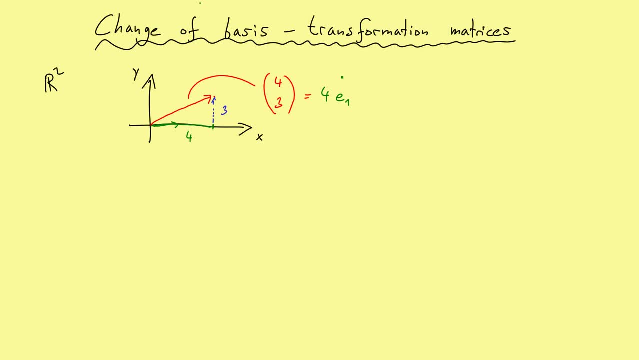 just this vector arrow and we go upwards. These are three steps in the second direction. This would be this arrow here. So this is E2.. If we choose the basis in this way, we call it the canonical basis or just standard basis. Therefore, this is just and this is So very easy. 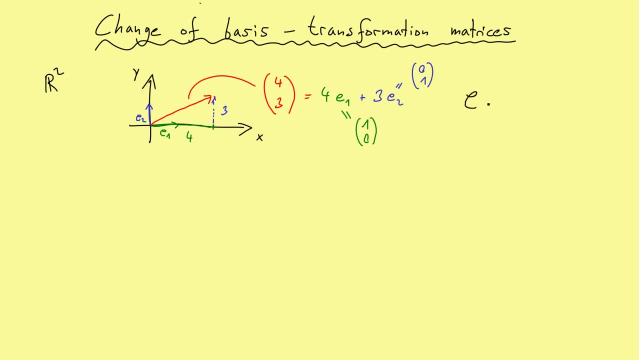 vectors and the canonical basis would be now we call it C for canonical and And then we put the first vector this is and there we have, or just with our notation here, e1 and then e2.. However, maybe we have a problem where it's good or better to switch between the canonical basis here and a better chosen basis. 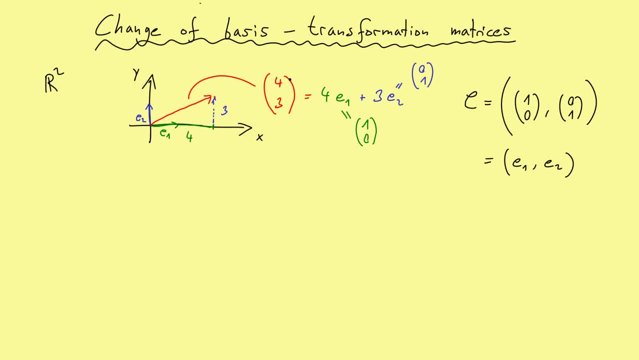 For example, if we have this vector for 3, so this direction as an important direction in our problem, So, for example, everything goes more or less in this direction, Then it would be good to choose the basis with one vector in this direction. 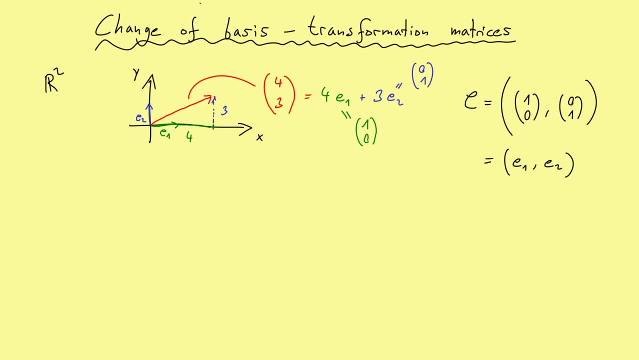 So maybe we choose for 3 as a basis vector and then another one, for example, we are only independent, of course. then we have a basis. For example, we choose this, Then let's call it just b1 here and b2 the other one. 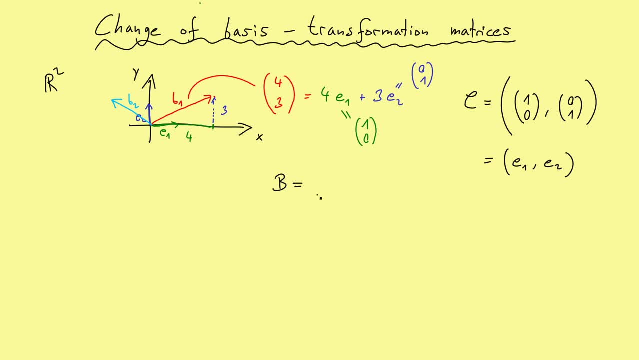 Then our new basis. we call it b, that's just the vector b1 and b2. And in this new basis we measure how many steps we have to go in the b1 direction here. So if everything is in the b1 direction, maybe our problem is constructed in this way. 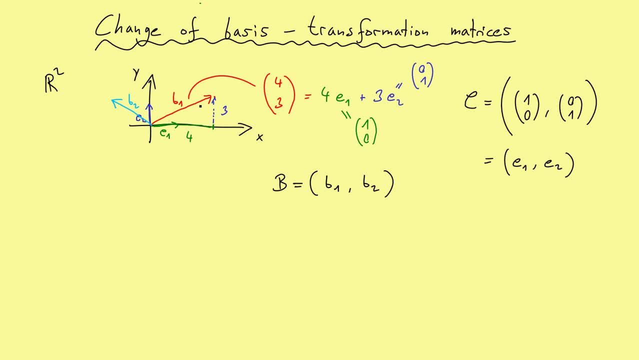 Then we have to say, okay, one, two or three steps in b1 direction. So maybe one step in the b1 direction would be this vector for 3.. But in the new basis b1, and this is the red one here- 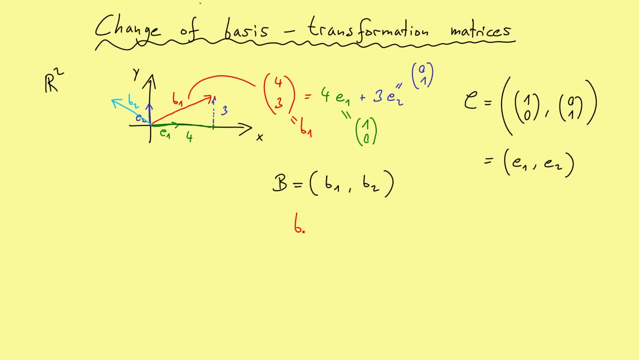 This is b1.. In our new basis b1 would be just 1, 0.. And then I say it's in the basis b here, And then we are not confused with the other notation. So we could write here the canonical basis c to distinguish between the two. 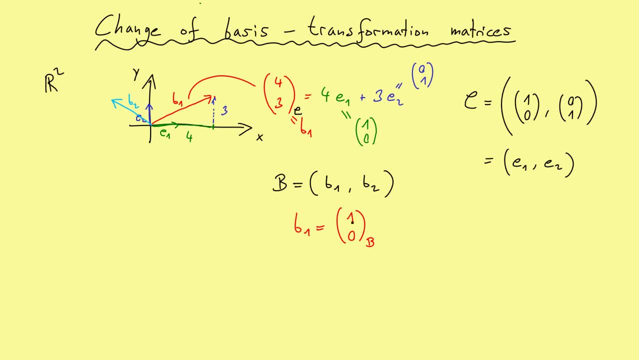 But here it's important. Then we say it's measured in the basis b. So one step in the x direction, in the new x direction, Would be just going from there to there, And this is just the vector b1. But now measured in the new basis b. 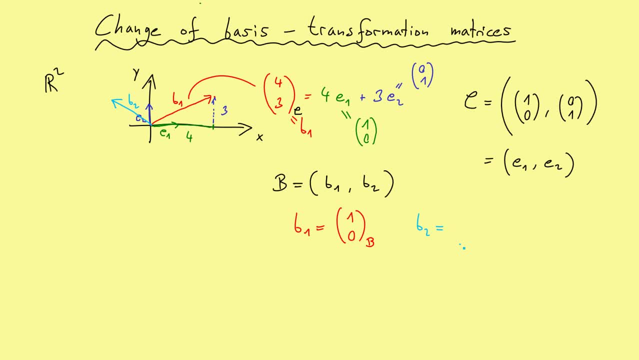 Of course the same holds for the vector b2.. This would be another, So just the other one. So 0, 1 measured in the basis b. So now it's important: how can we switch between these two basis, Or maybe we have more than one basis? 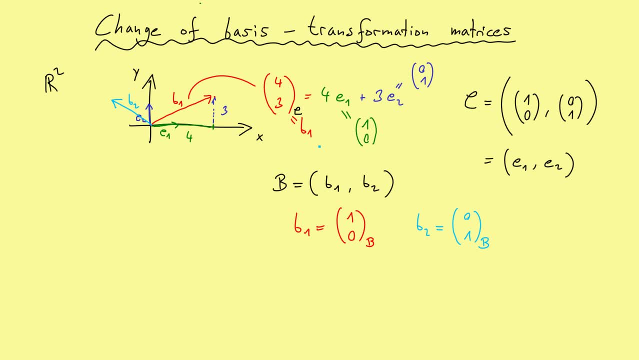 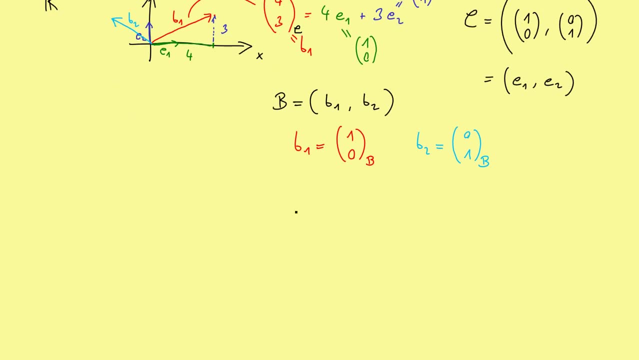 Then we have to know how to easily switch between two of them. A good thing is here to imagine the following picture. So we start by the vector space R2.. Just think of this vector space R2 as the abstract vector space, So this one where we live in. 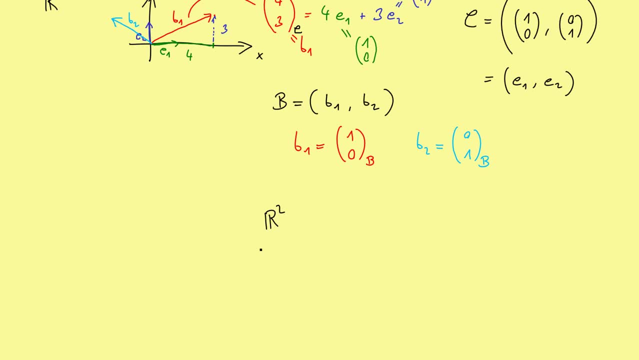 And to describe it we will choose a basis. So, for example, choosing a basis in the canonical way Would mean we say: maybe we call it phi index c And this is the canonical basis. And now we have R2 with this basis c here. 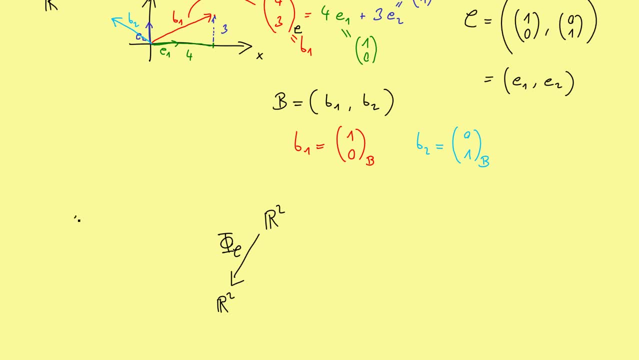 What do I mean by that? So it's easy, Since I have now my basis chosen as e1 and e2.. So these are these vectors above, So e1 here and e2 in the y direction. Then I say, okay, e1 is sent to the first basis vector. 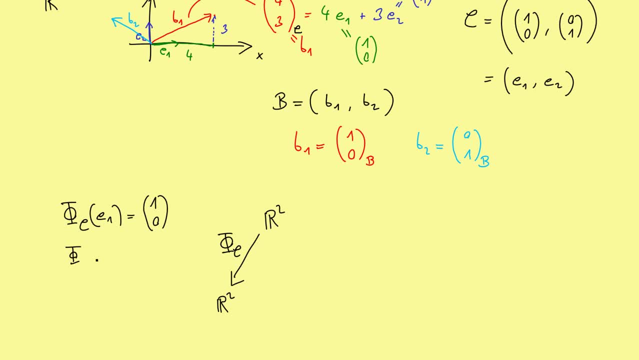 So 1, 0.. And e2,. so this is c, e2 is sent to the other one, 0, 1.. So indeed it doesn't change anything, It's just the identity when I see R2 as the basis vectors as well. 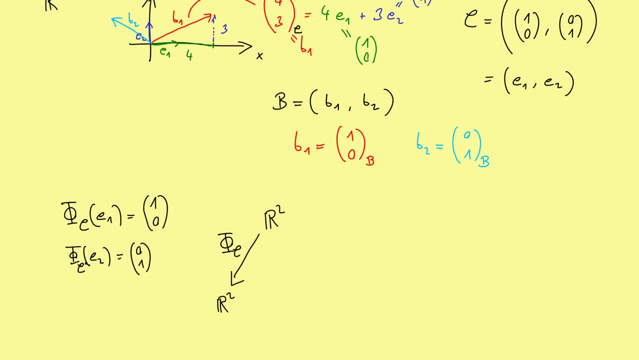 But when. I will choose another basis and this is important now. So now we go in the basis b, So I call it phi b, And also in R2.. Now this R2 is measured in the basis b, So this means I have my phi b acting on the vector b1 here. 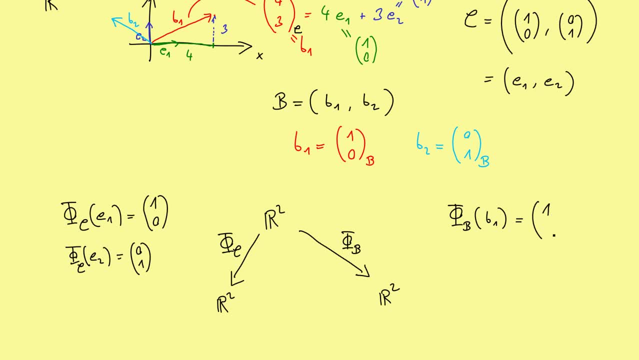 And this vector is sent again to the first unit, vector 1, 0. And the second one. so phi b2 is sent to 0, 1.. So this is the same as above here, But of course this is just R2.. 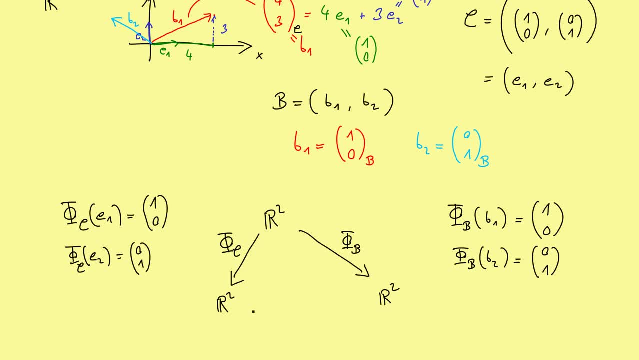 And this is R2.. The one thing that is changed now is what vectors do we describe. So we want to describe the same vectors but in different basis. Therefore we will add again the basis as an index. Then we know which vectors may coincide here. 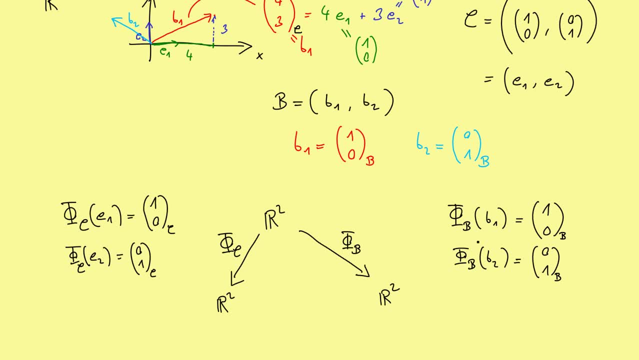 Okay, but this is just a description. So we describe the vector b1 in the basis b And that is very easy for b1.. b1 in the basis c looks different, So this is 4, 3 in this basis. 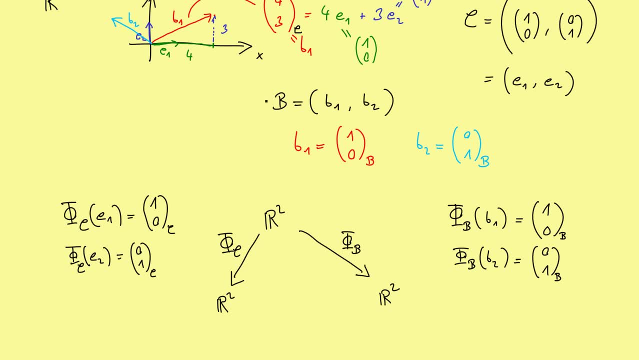 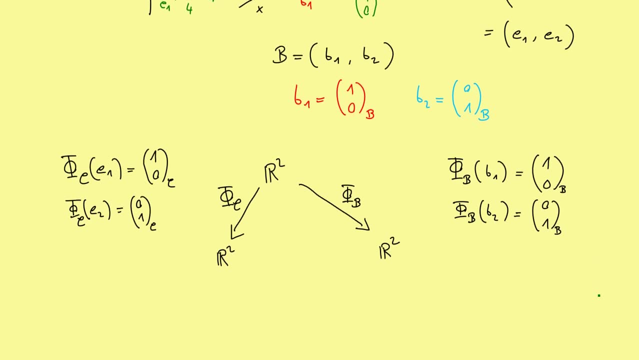 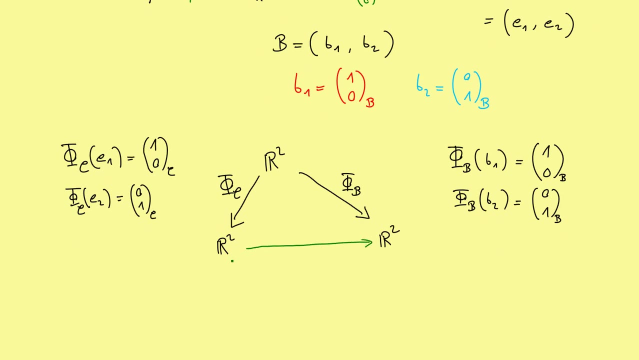 So it's much more complicated. The important part is now, of course, how do we switch between these two? So this is just a map that we can draw here. So we start by R2 that have the basis c And go in R2 that have the basis b. 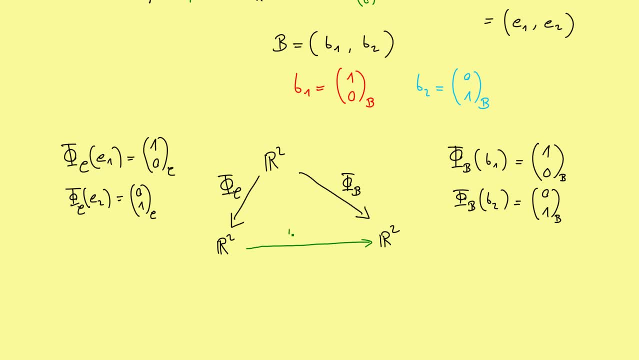 So we can call it a transformation matrix. So we go from c to b, So I will rotate in this way. Therefore, this is the linear map that let us switch between the basis c and the basis b of the vector space, And if we want to go from b to c, we have the transformation matrix. b goes to z. 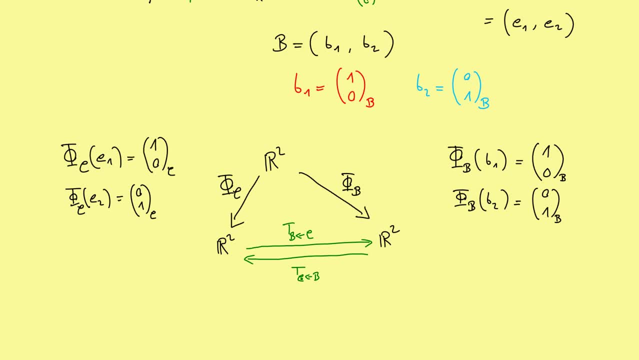 Of course, this is just the inverse matrix of this matrix, or the inverse map. Maybe I should switch the color here And then we can calculate what is t, c to b. So okay, this is just going the errors. So we have. first we start here. 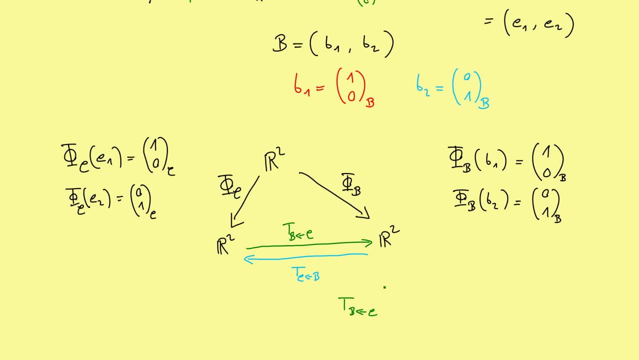 Then we have the inverse of this linear map that we called phi index c, But it was just identity matrix, So in this case it is not so important. But we could have another basis here. So the basis c could be just maybe b1 and b2 here. 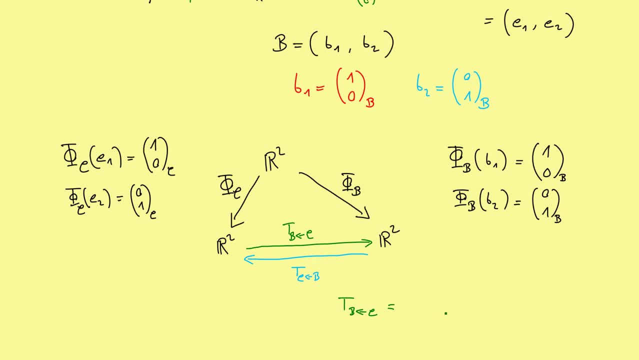 Then it is important to have it, So I write it down in this way. So we start with the inverse of this map And then compose it with the next one, And this is phi b. In the same way we get the matrix. 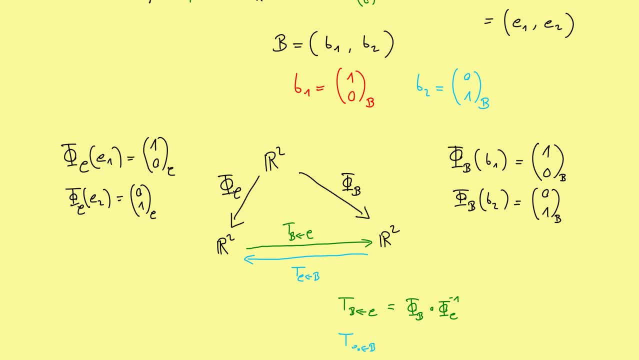 That goes from the basis b into the basis c. So this is now first the inverse of phi b. So we start from right to left, This inverse, And then we go just phi c. So this is just the composition of the map. 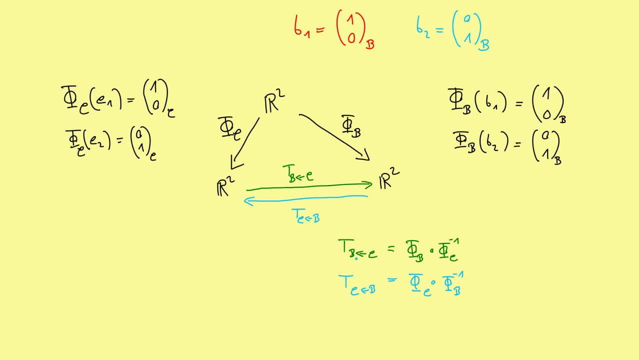 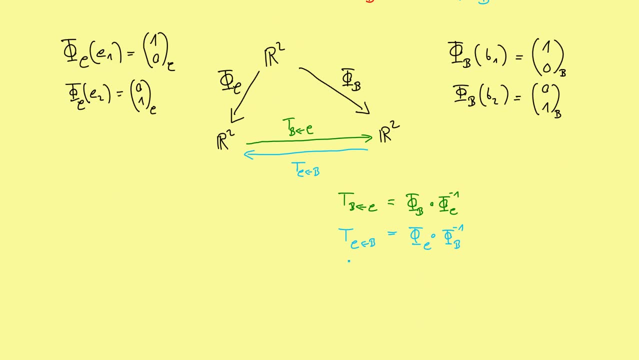 So nothing happened here. But it is good to know what we do, And now I can show you how to calculate these transformation matrices. So we start with the easy one, That would be, start by the basis b and go into the canonical basis. 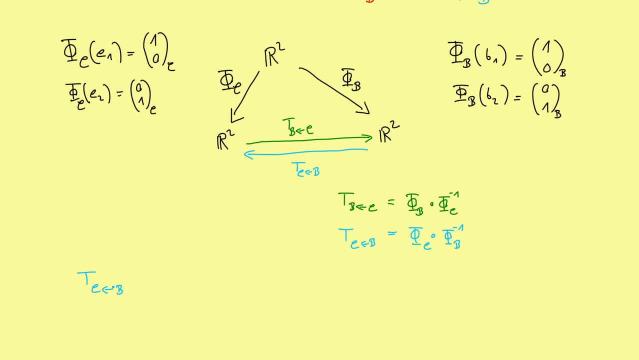 Since we already know how the vectors look like in the canonical basis. So now we can see how to do it. So to get the first column of a matrix We have to act the matrix onto the vector. Of course this is now in the basis b. 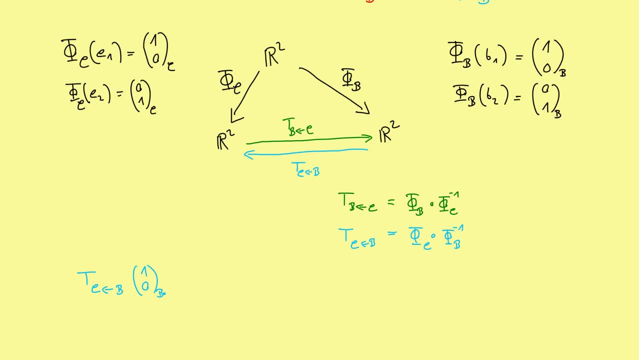 So I could say maybe this is in basis b, But of course this is clear, since we start in this R2.. We have the basis b chosen on this R2.. Okay, and this means that we have phi c. So this is the c and phi b inverse. 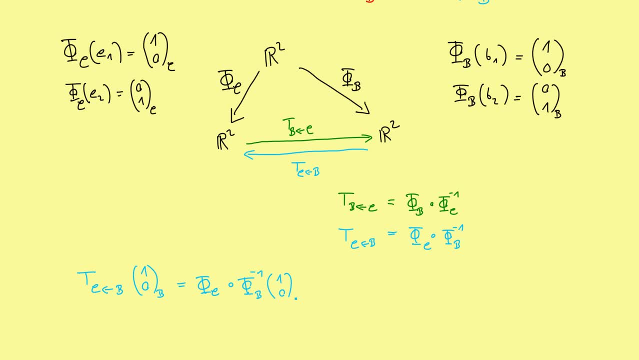 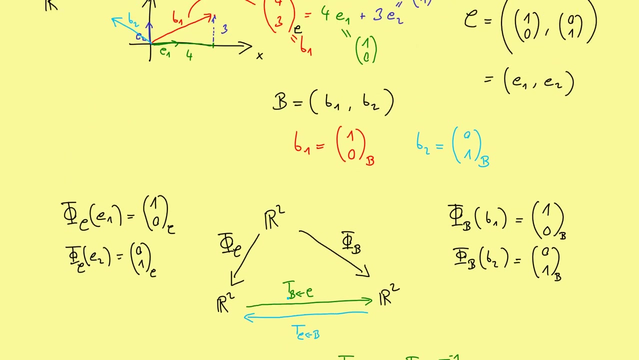 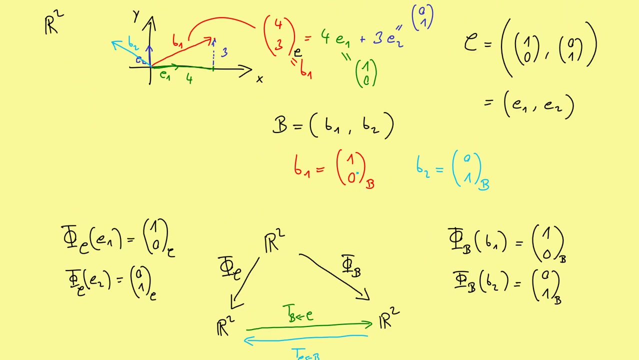 And now we have here the vector: Okay, but what is the inverse phi b acting on? So when we can scroll up And then we see: Ah, okay, 0,, 1 is b 1.. So the basis b is our vector b 1.. 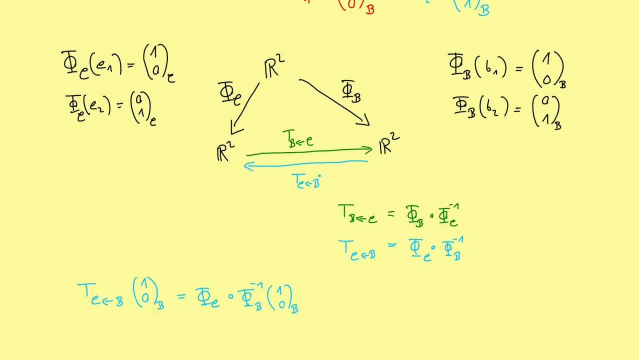 That means our phi b inverse. here is just our vector b 1. In this vector space, Therefore, we have phi c of this vector b 1.. Okay, but this is just how does b look like in the basis c, So in the canonical basis. 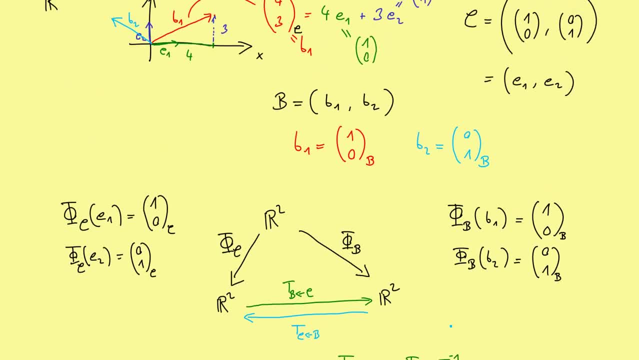 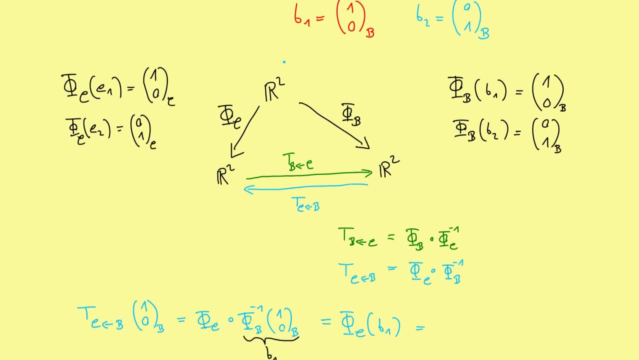 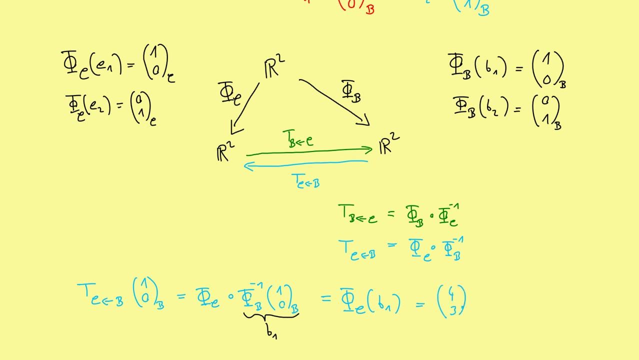 And we already know this, since b 1 was chosen as 4.. So you can see it here: 4, 3.. And this is just the representation in the basis c, So in the canonical basis. So we have 4, 3 here. 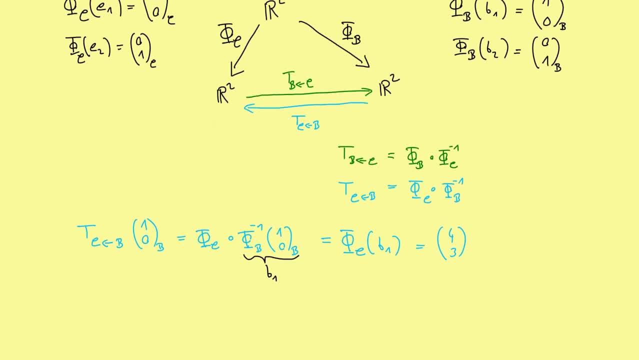 Okay, and the same we can do for the second one. So the second vector would be just 0, 1.. Okay, and put in the basis b, But we know that we calculate in this R2.. So we could omit this in this calculation. 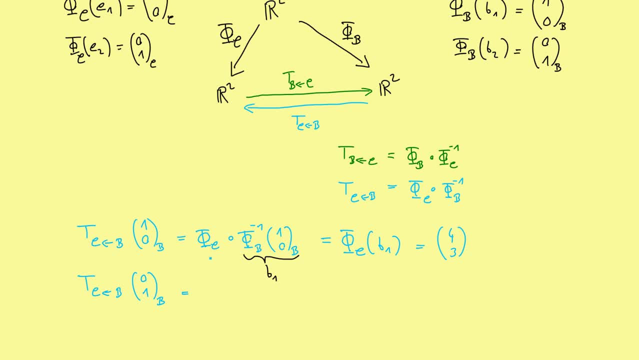 Since we've chosen the phi's, So the phi's define what we do. Okay, but this is the same. Then we have phi c in the end of b 2. So this is the canonical representation of b 2. Just in the standard basis c. 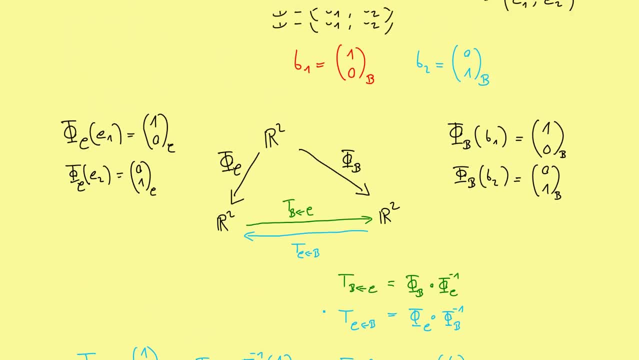 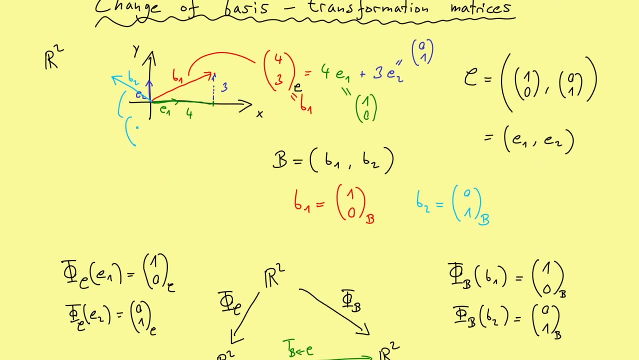 Of course I didn't say at the beginning What b 2 should have been, So the picture suggests that we have here just the vector Minus 2, minus 2, for example, So what b 1 and b 2 are chosen. 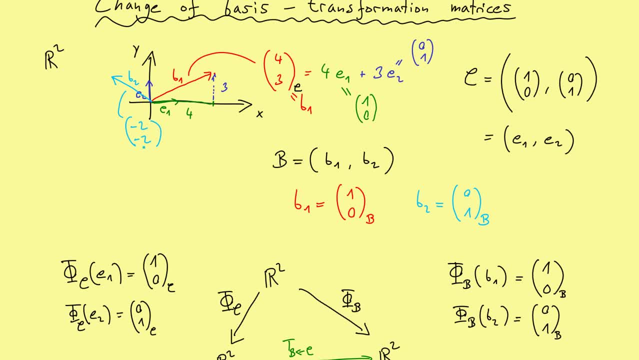 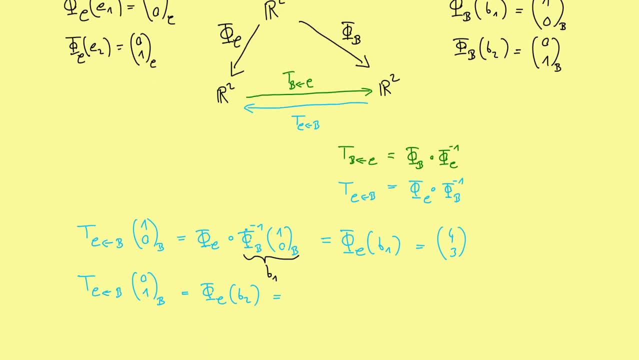 So b 1 was fixed and b 2 was also fixed, But now I have the numbers here. So minus 2 and minus 2.. And this is the solution here. So we have again minus 2, minus 2.. 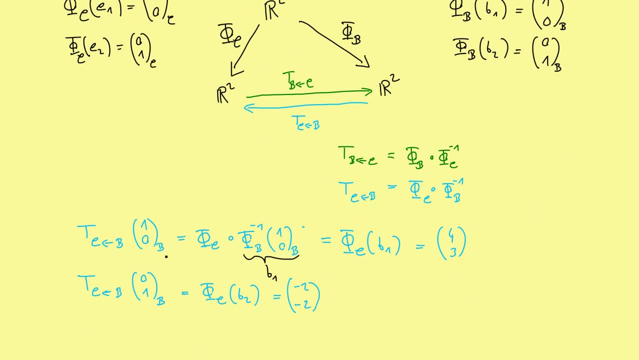 Okay, now we know what the matrix does on the standard basis, So to say. Then we know the columns. So from these two we know that the matrix t, coming from b and goes to c, Is just the matrix with the first column for 3.. 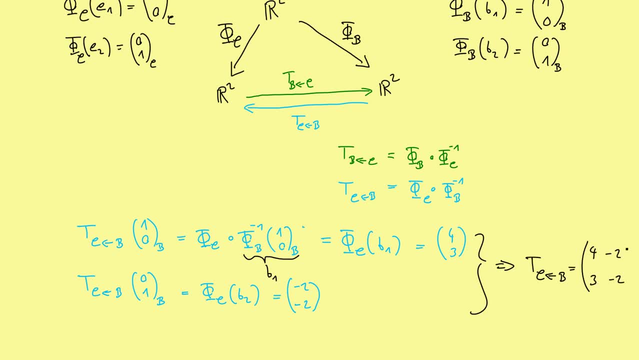 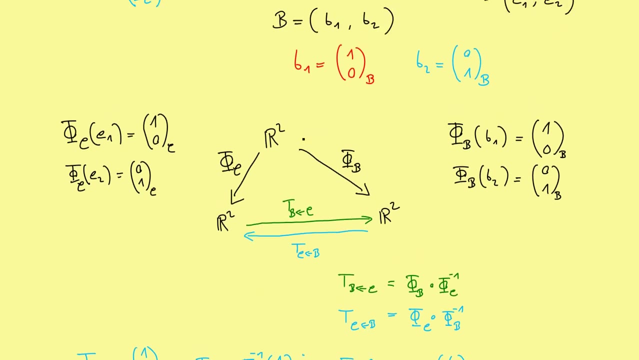 That is this one, And minus 2,, minus 2.. And this one- Okay, I see this was a long explanation- Just for saying, Okay, you need the transformation matrix from b to the canonical basis. Then just put in the canonical representation of the two vectors. 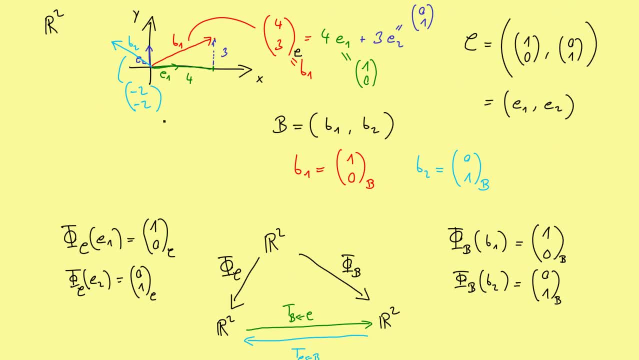 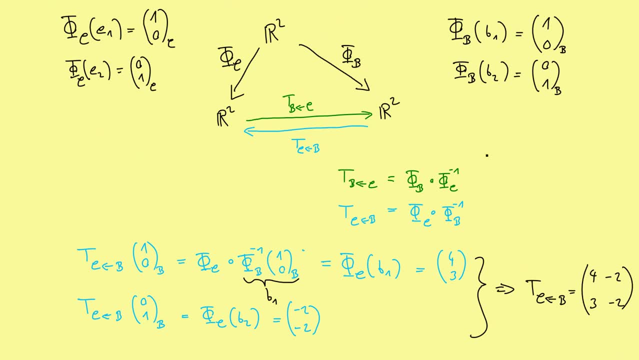 So for 3 here and minus 2, minus 2 here, Put them in the columns of the matrix. But this was the explanation why we do this. Then we go from the basis b here to the basis c By doing the matrix multiplication as usual. 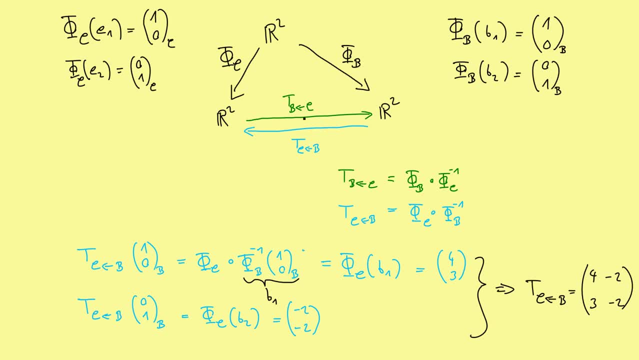 But if we want to go the other way- And that is usually what we want to do, We want to go from the canonical basis into the new basis- Then we have to invert this matrix. Okay, now we can say: If we want the basis, 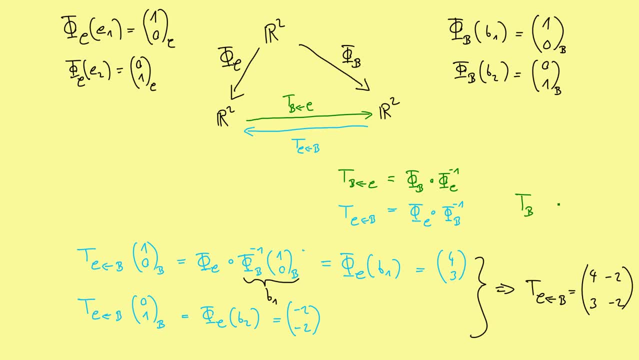 The transformation basis change here, So the transformation matrix That goes from the canonical basis c and to the new basis b. We have to invert this transformation matrix That is given by the two column vectors. So maybe I just write it in this way. 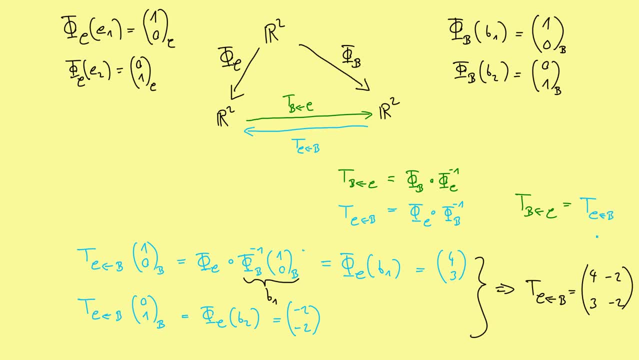 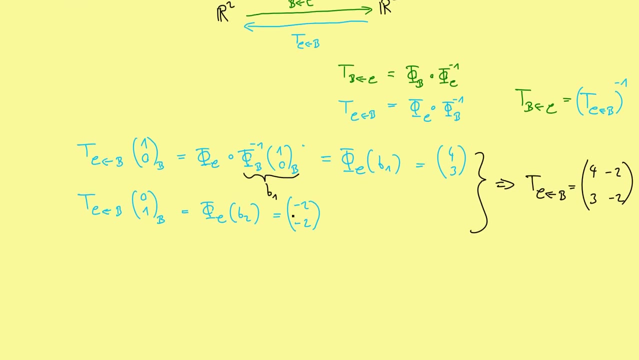 We can get this transformation matrix very easily, But we have to invert it. So the inverse of this matrix gives us the wanted transformation matrix. Obviously, I hope that you can do the inverse of a matrix, So I will skip the calculation And just tell you the solution. 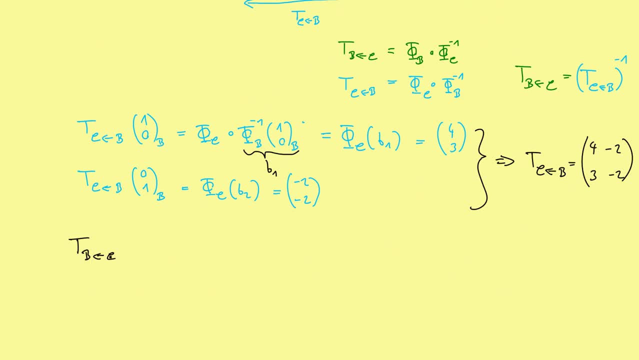 So the matrix c to b is the inverse of this matrix, here Minus two minus two, Inverse, And the solution is just one, three half here Minus one minus two, And then we have the transformation matrix Going from the canonical basis into the new basis. 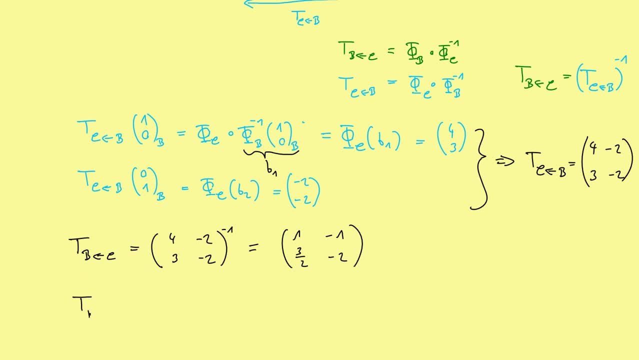 And we can check it And just look at the new basis vectors, Then we should get one zero and zero one, as always. So putting in here our first one, This is four three, So this is b one. And then putting: So this is the canonical basis. 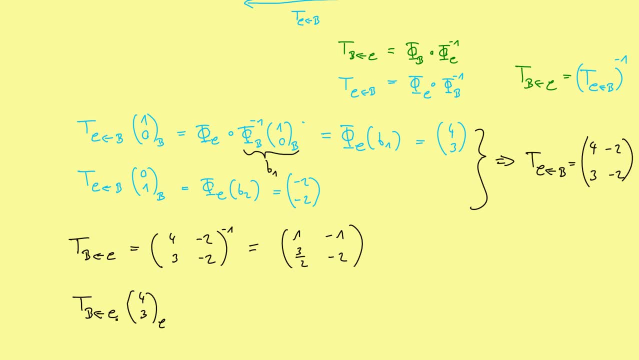 Of course we won't put in the canonical basis on the right hand side, And then we get four minus three, And here we have six minus six And as you can see, So this would be now in basis b, As we see here. 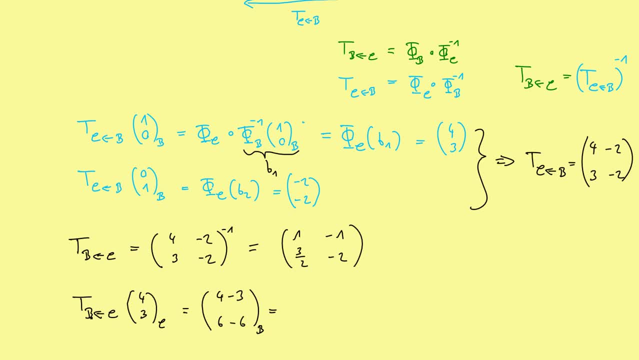 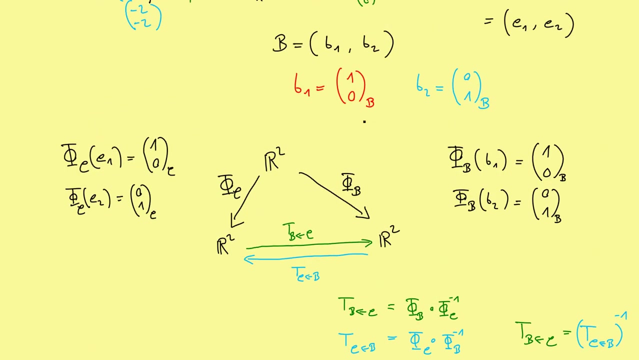 Putting in the basis c And getting a vector in the basis b. So this is one zero in the basis b And that is what we know from the beginning. So we know how we run should be one zero in the new basis. So this is correct. 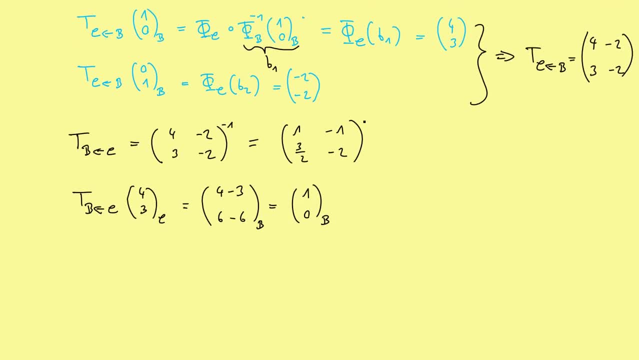 And now we can transform every other vector in the new basis. For example, if you get a vector, Say what is the vector three, two in the new basis b, Then you can just put in the matrix in front of the vector And do the matrix multiplication.